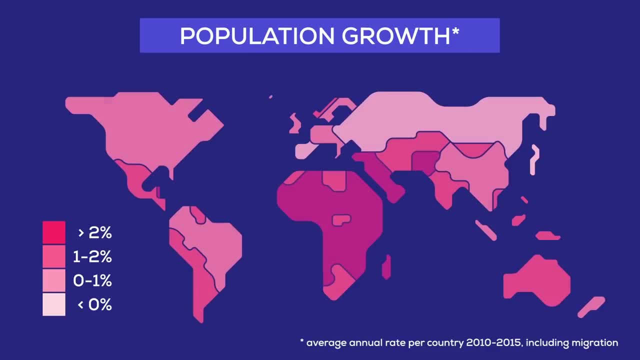 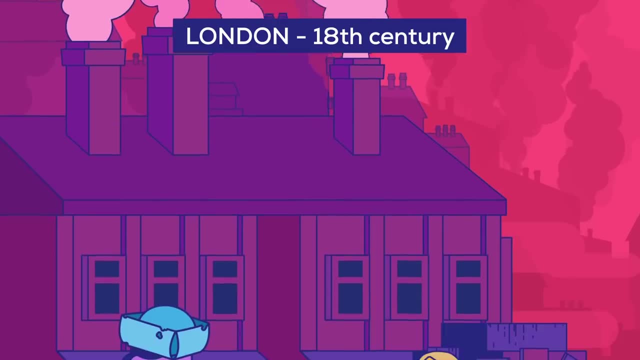 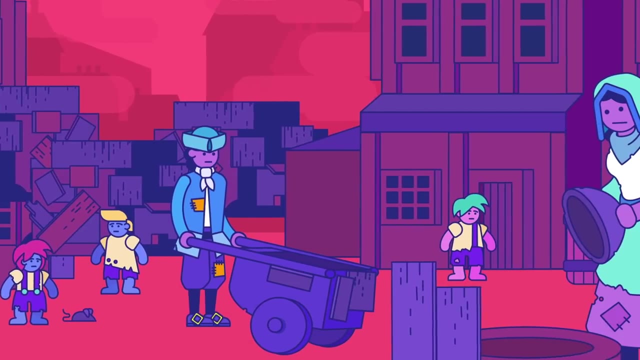 The demographic transition. Most developed countries have already made the transition, while other countries are doing it right now. Let's go back to the 18th century, when the entire world, including Europe, was in the first stage of the demographic transition. By today's standards, Europe was worse off than a developing region. 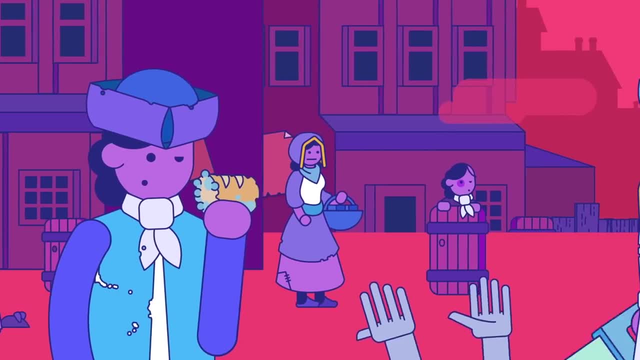 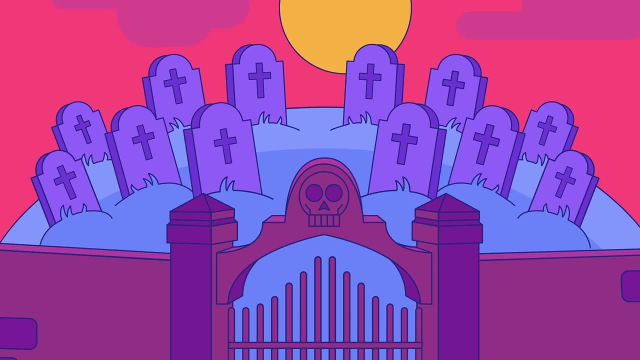 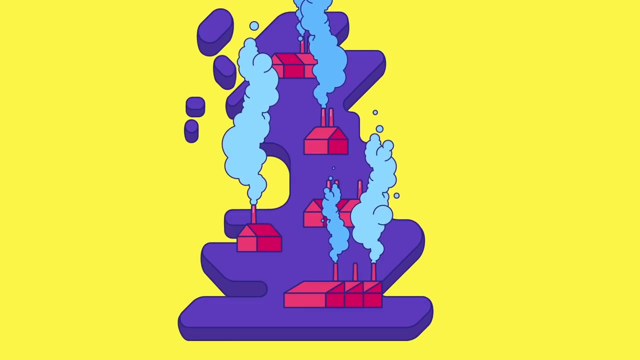 suffering from poor sanitation, poor diets and poor medicine. A lot of people were born, but lots of them died just as fast, so the population hardly grew. Women had between four and six children, but only two of them would reach adulthood. Then the Industrial Revolution happened in the UK. 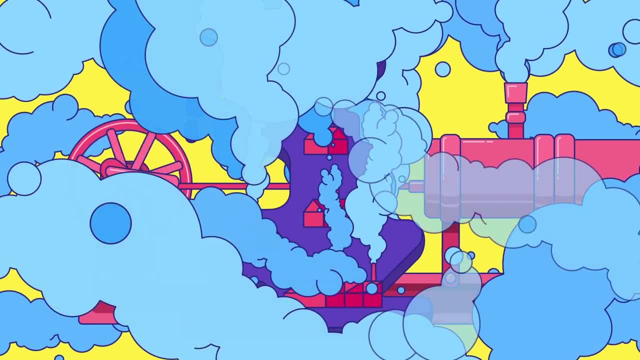 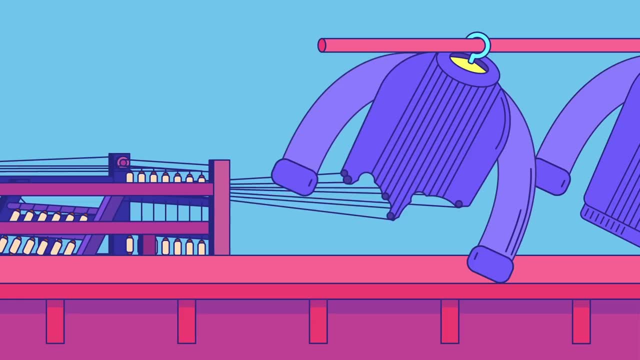 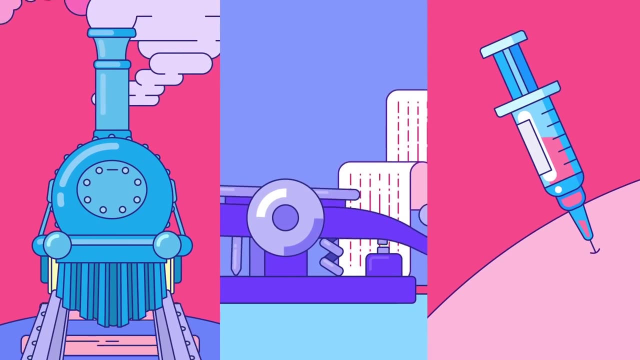 and brought the greatest change in human living conditions since the agricultural revolution. People went from being peasants to workers. Manufactured goods were mass produced and became widely available. The sciences flourished and advanced transportation, communication and medicine. The role of women in society shifted. 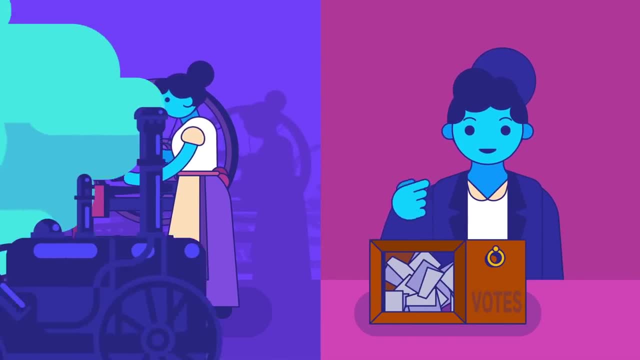 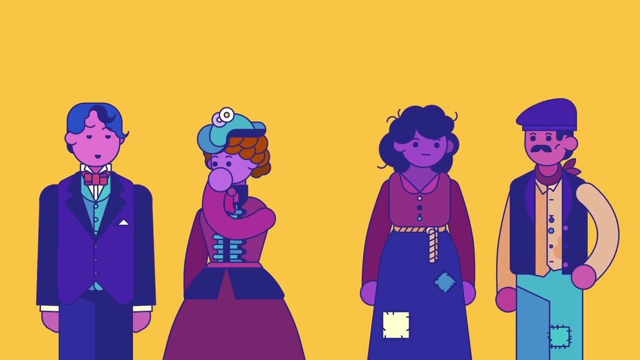 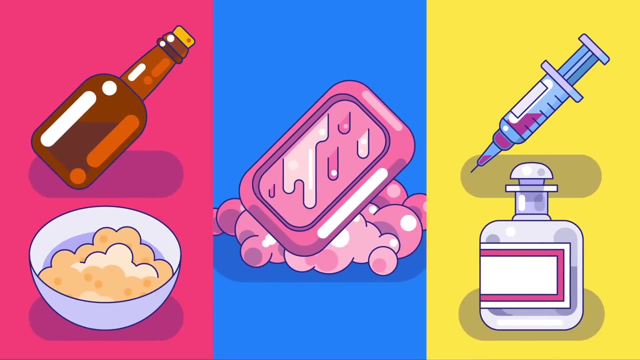 and created the conditions for their emancipation. Slowly, this economic progress not only formed a middle class, but also raised standards of living and healthcare for the poor working population. The second transition stage started. Better food supplies, hygiene and medicine meant people stopped dying all the time. 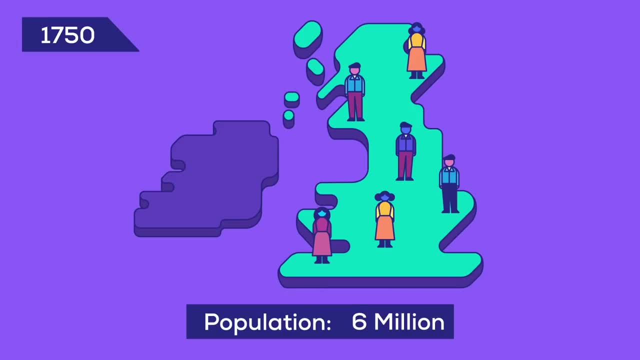 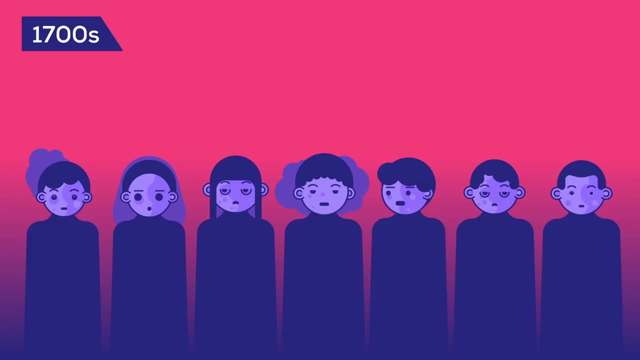 especially so at a very young age. The result was a population explosion, doubling the UK's population between 1750 and 1850.. The main reason families used to have lots of children was that only a few of them were likely to survive. 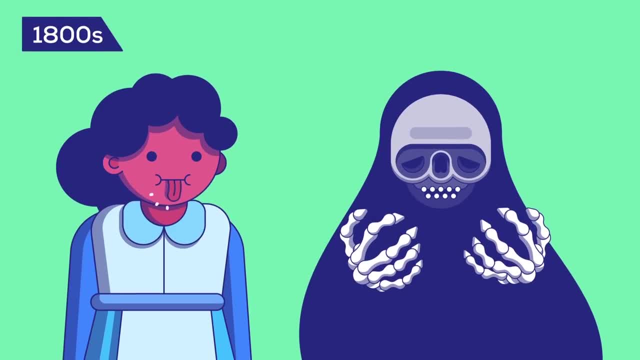 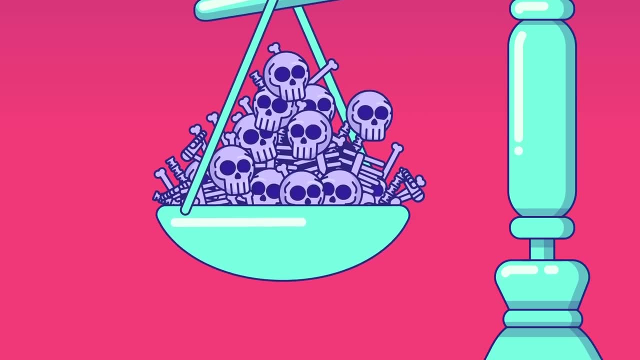 Now that had changed. so the third stage of the transition was set in motion. fewer babies were conceived and population growth slowed down. Eventually, a balance emerged: Fewer people were dying and fewer children were born, so the death rate and birth rate became stable. 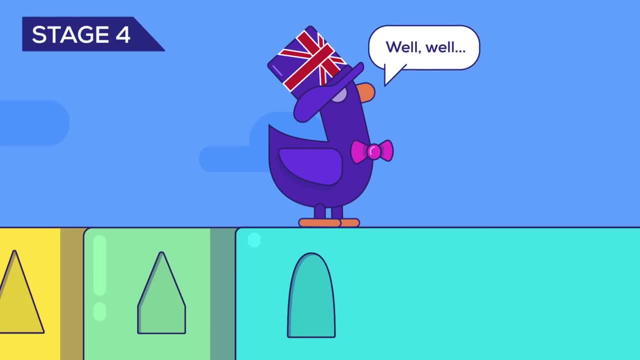 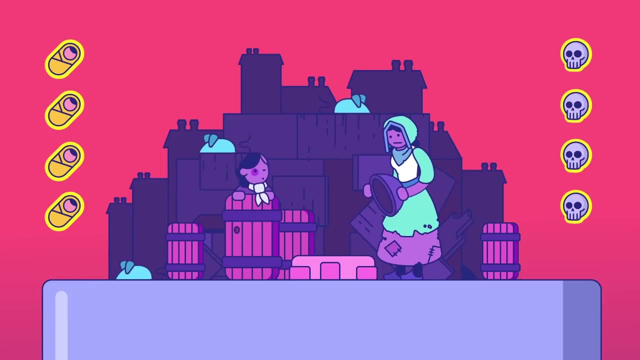 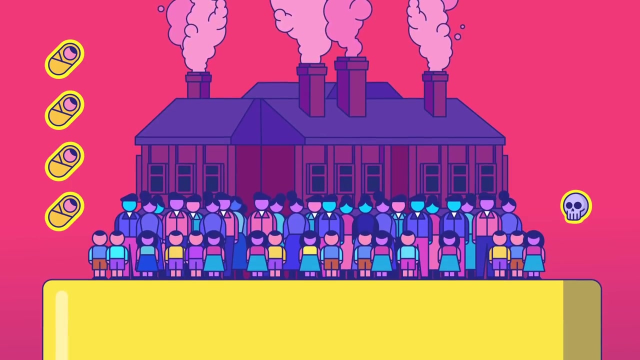 Britain had reached the fourth stage of the demographic transition. This didn't only happen in the UK. More and more countries went through the four stages. First: many births and many deaths due to bad living conditions. Second: better living conditions leading to fewer deaths and a population explosion. 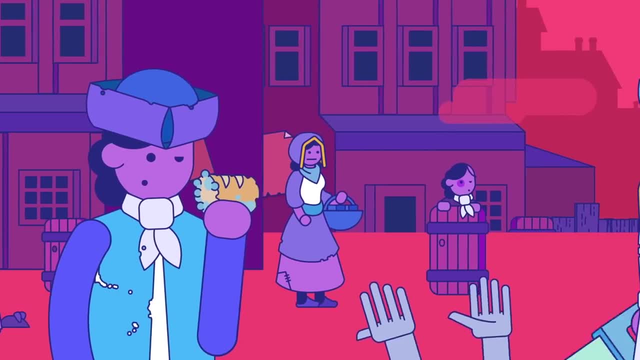 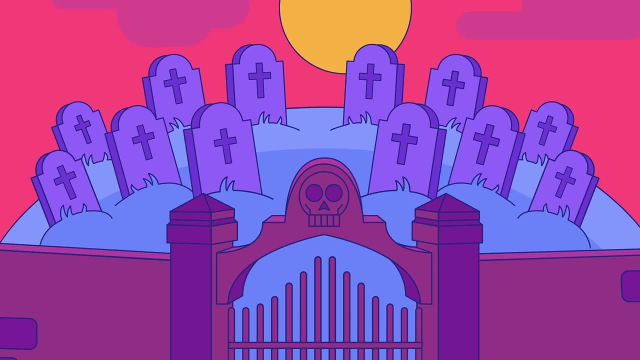 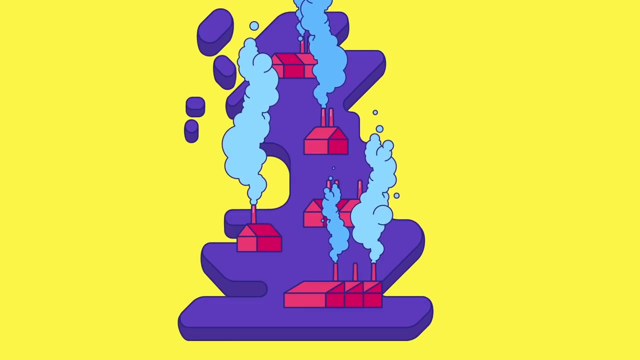 suffering from poor sanitation, poor diets and poor medicine. A lot of people were born, but lots of them died just as fast, so the population hardly grew. Women had between four and six children, but only two of them would reach adulthood. Then the Industrial Revolution happened in the UK. 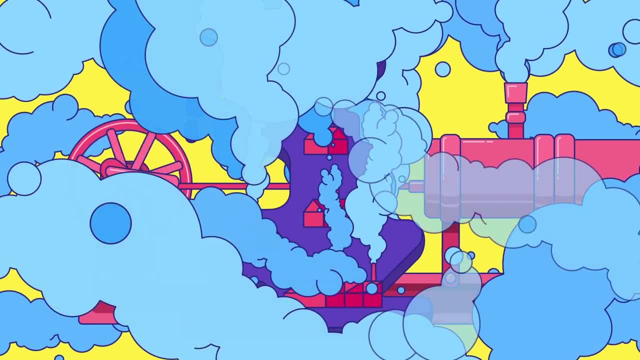 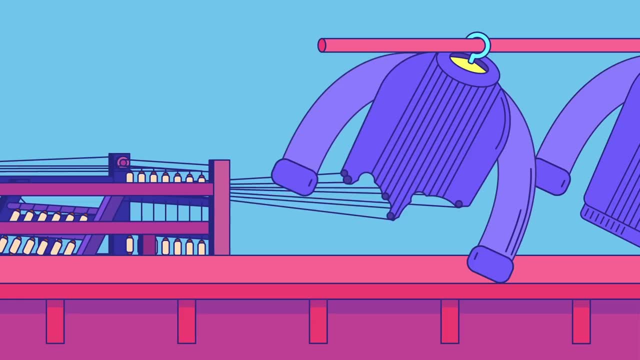 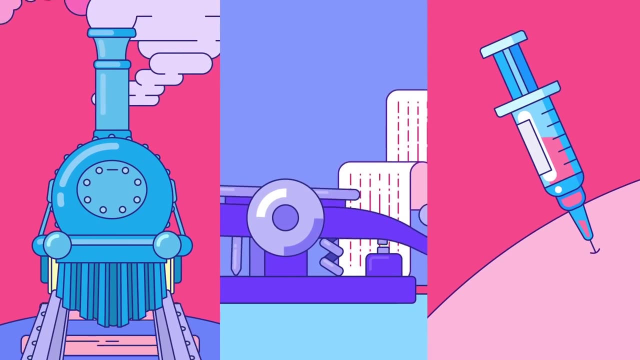 and brought the greatest change in human living conditions since the agricultural revolution. People went from being peasants to workers. Manufactured goods were mass-produced and became widely available. The sciences flourished and advanced transportation, communication and medicine. The role of women in society shifted. 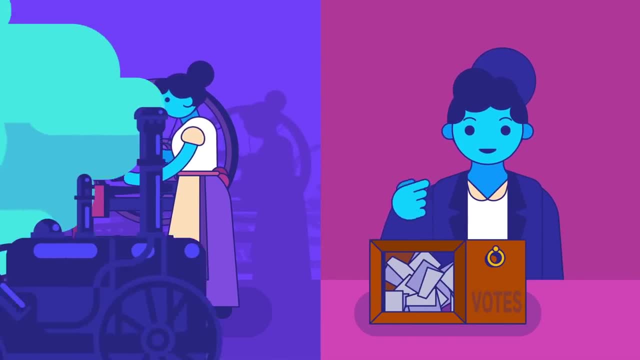 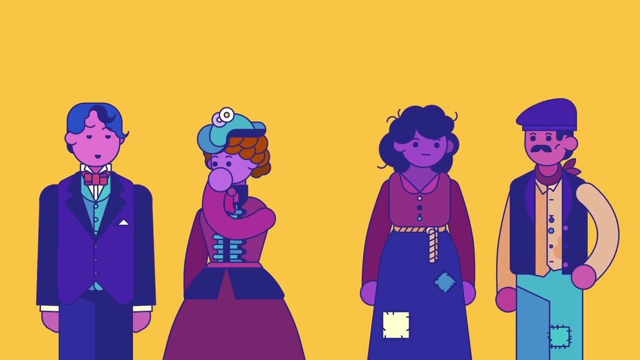 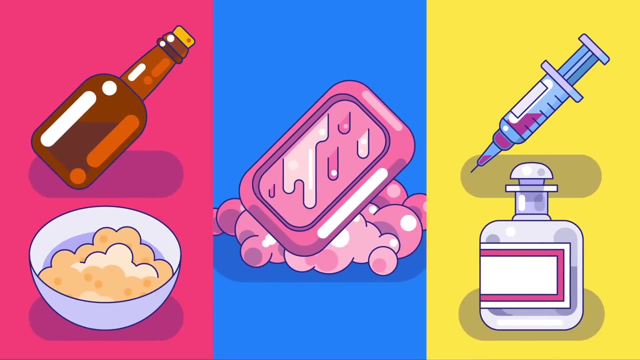 and created the conditions for their emancipation. Slowly, this economic progress not only formed a middle class, but also raised standards of living and healthcare for the poor working population. The second transition stage started. Better food supplies, hygiene and medicine meant people stopped dying all the time. 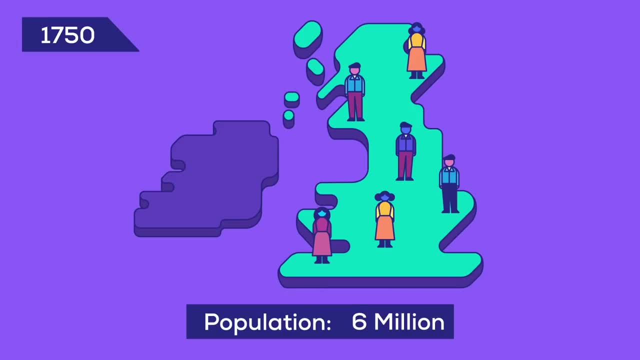 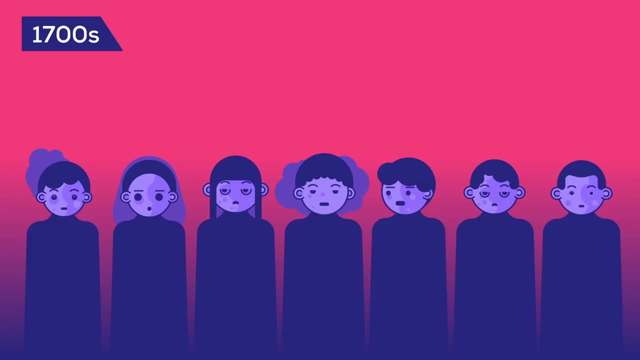 especially so at a very young age. The result was a population explosion, doubling the UK's population between 1750 and 1850.. The main reason families used to have lots of children was that only a few of them were likely to survive. 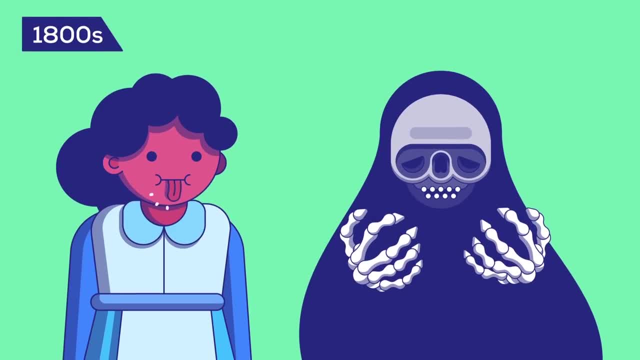 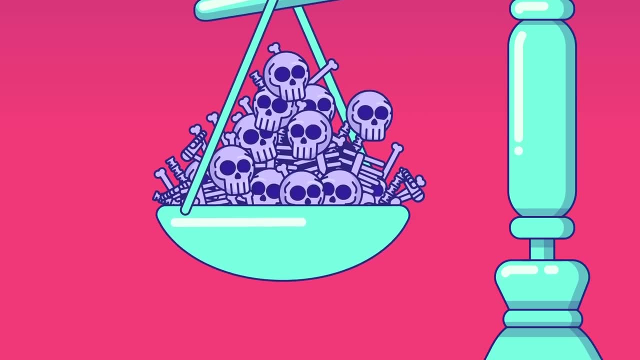 Now that had changed. so the third stage of the transition was set in motion. fewer babies were conceived and population growth slowed down. Eventually, a balance emerged: Fewer people were dying and fewer children were born, so the death rate and birth rate became stable. Britain had reached the fourth stage of the demographic transition. This didn't only happen in the UK. More and more countries went through the four stages. First: many births and many deaths due to bad living conditions. Second: better living conditions leading to fewer deaths and a population explosion. 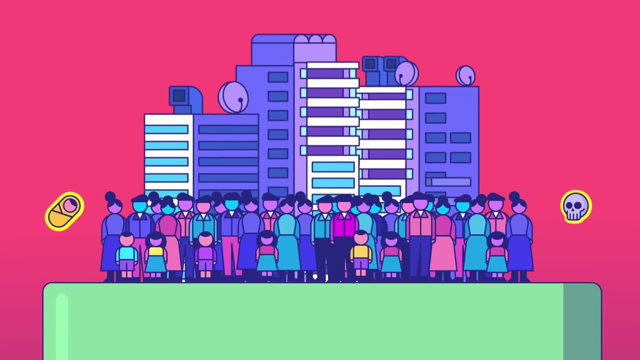 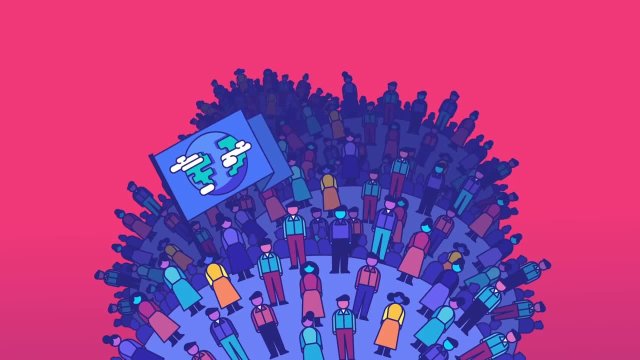 Third, fewer deaths resulting in fewer births, and population growth came to an end. But if birth rates have dropped so much, why is the population still growing so fast? Well, the children born in the population explosion of the 70s and 80s. 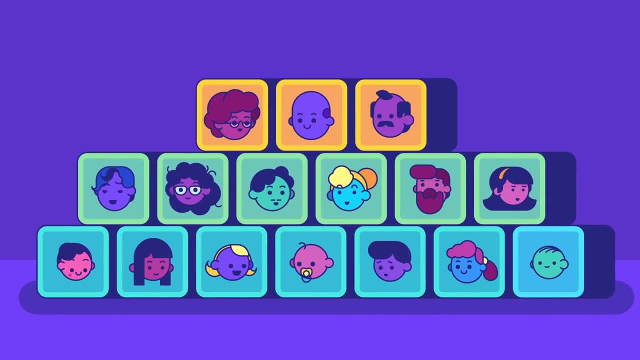 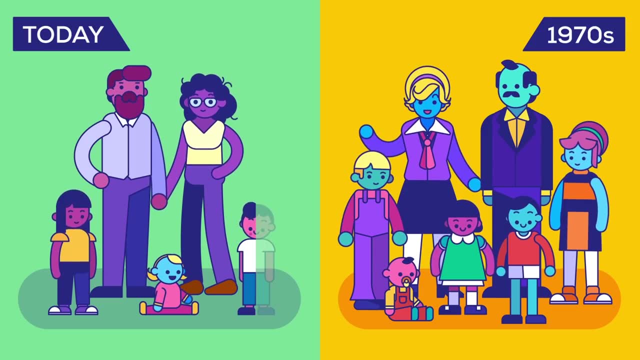 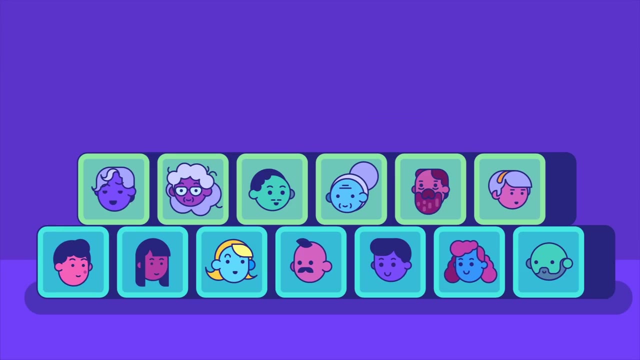 are having kids themselves now, leading to a noticeable spike in overall population, But they are having far fewer children on average than their parents. The average today is 2.5.. It was 5 40 years ago. So as this generation gets older and fertility declines further. 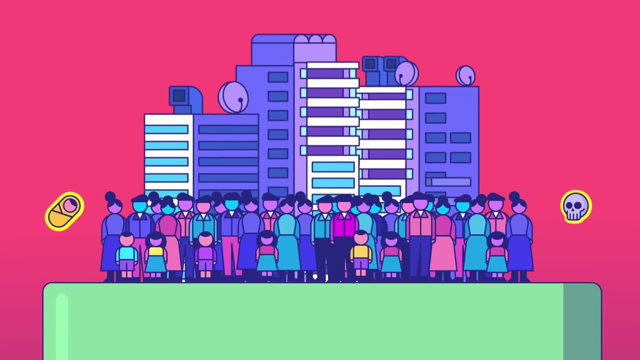 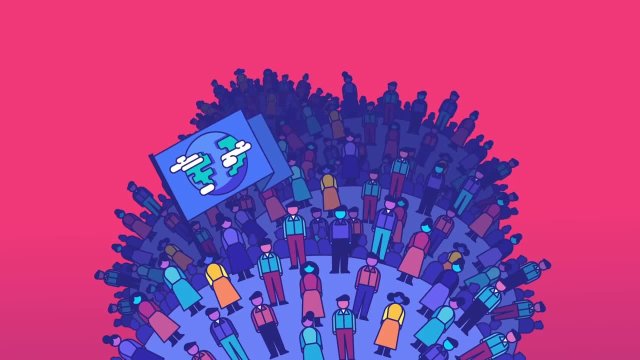 Third, fewer deaths resulting in fewer births, and population growth came to an end. But if birth rates have dropped so much, why is the population still growing so fast? Well, the children born in the population explosion of the 70s and 80s. 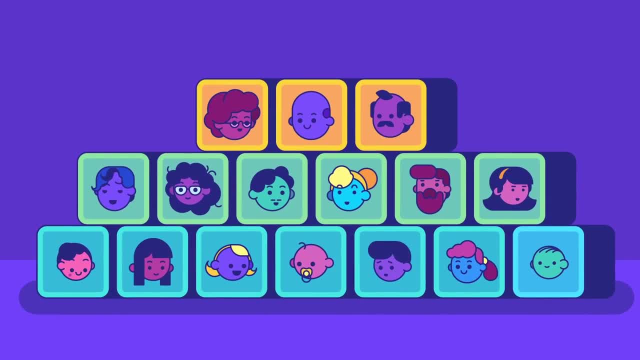 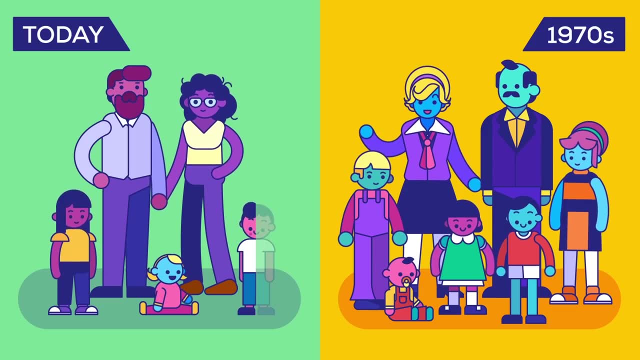 are having kids themselves now, leading to a noticeable spike in overall population, But they are having far fewer children on average than their parents. The average today is 2.5.. It was 5 40 years ago. So as this generation gets older, 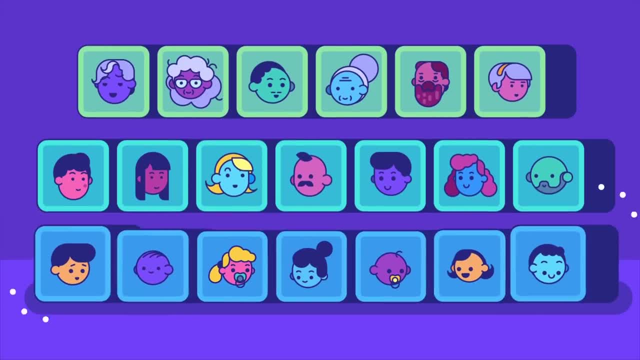 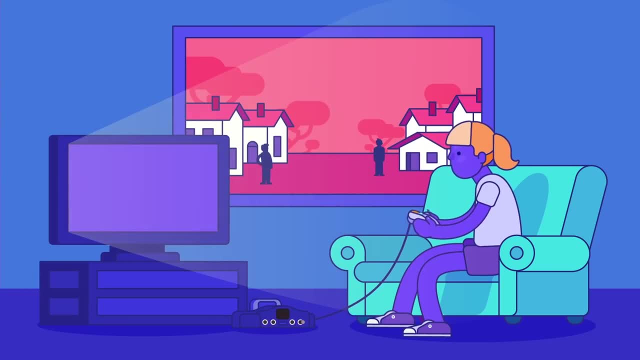 and fertility declines further, the rate of population growth will keep on slowing. This is true for every country. In the West, we tend to overlook progress in terms of population growth, But actually most of the world's countries have made it to the fourth stage. 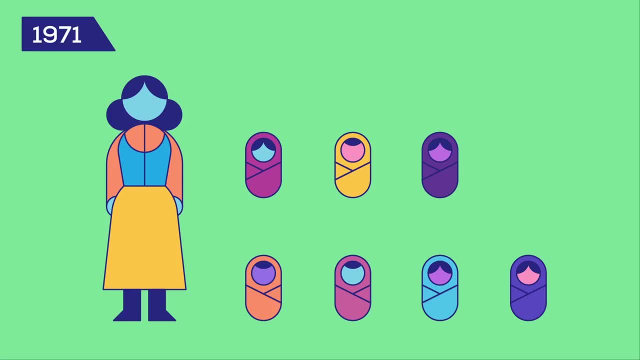 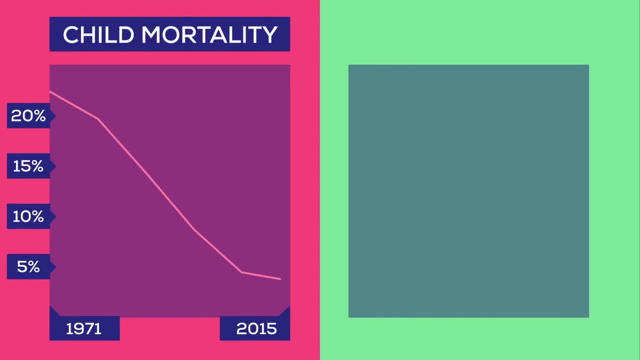 Just look at Bangladesh. In 1971, the average woman had seven kids, but 25% of them would die before the age of five. In 2015,, the mortality rate was down to 3.8% and women had only 2.2 kids on average. 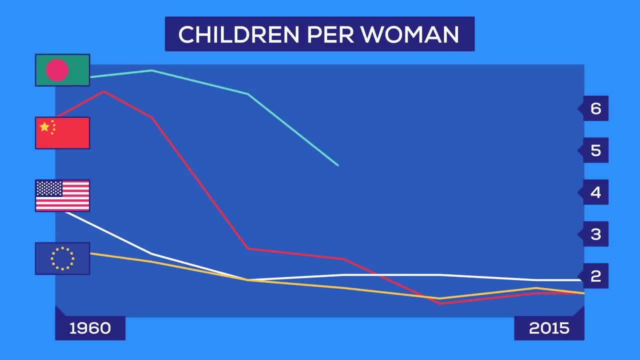 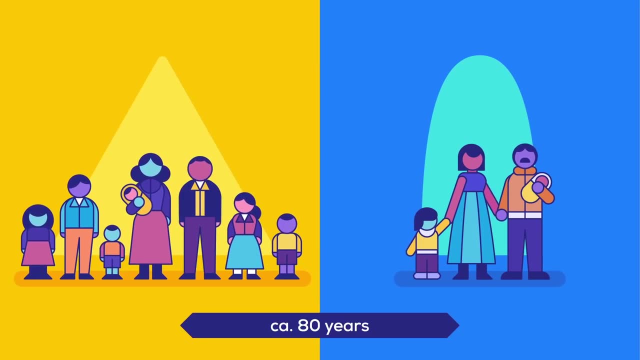 This is the rule, not an exception. We are not special, We just had a head start. It took developed countries about 80 years to reduce fertility from more than six children to less than three. Others are catching up fast. Malaysia and South Africa did it in only 34 years. 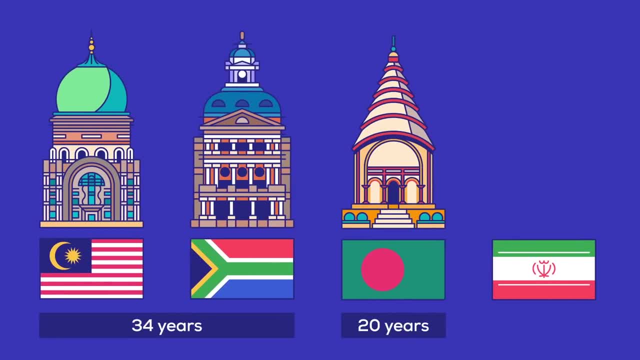 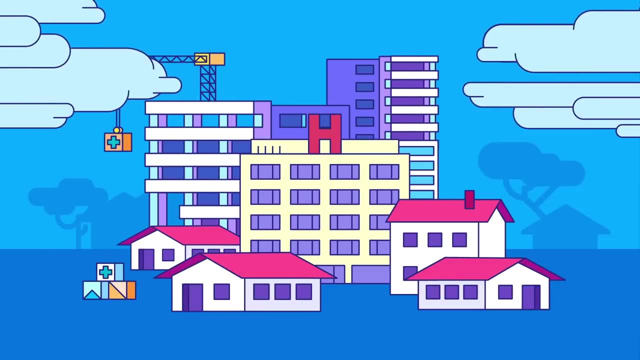 Bangladesh took just 20.. Iran managed it in 10 years. All these countries that are catching up didn't have to start from scratch, and the more support they get, the faster they catch up. This is why programs that help lower child mortality 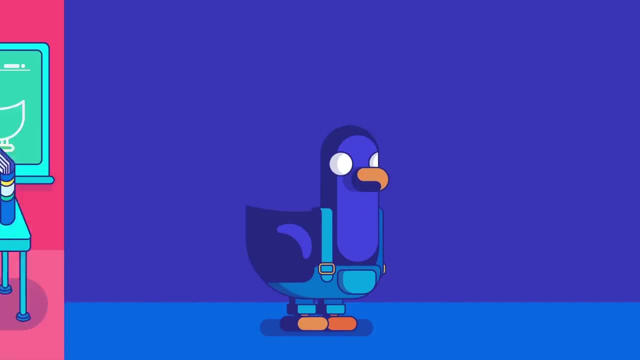 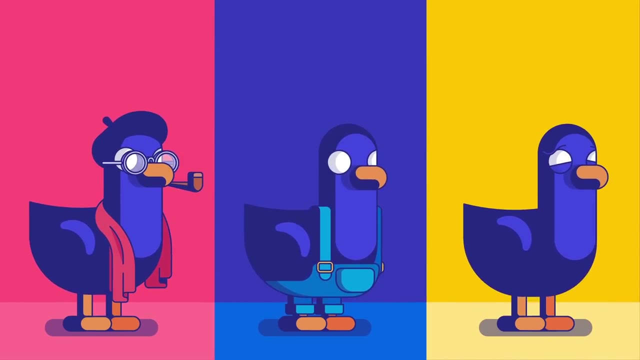 or help poor nations develop are so important. No matter what your motivation is- whether you dream of a world where all people live in freedom and wealth, or you just want fewer refugees coming to your country- the simple truth is that it's beneficial to you personally. 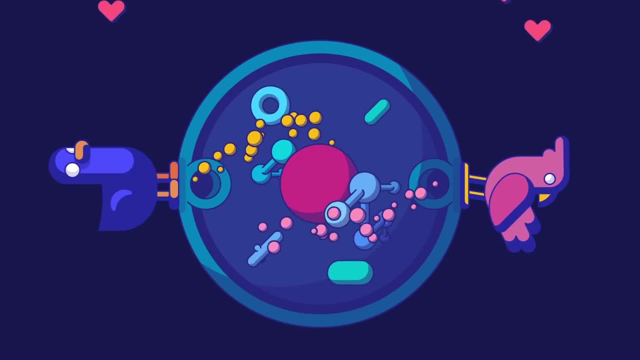 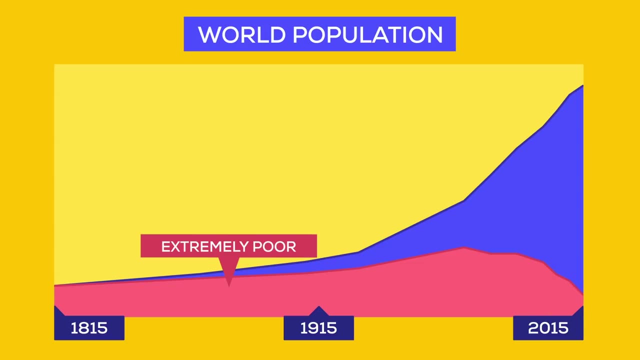 if people on the other side of the globe can live a good life. And we are getting there. The percentage of people living in extreme poverty has never been as low as today, So the future of global population growth is actually not an apocalyptic prophecy at all. 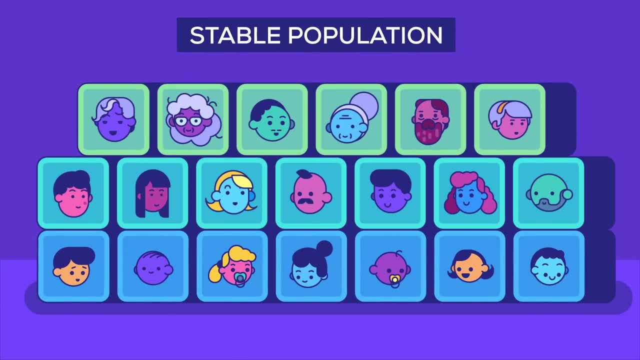 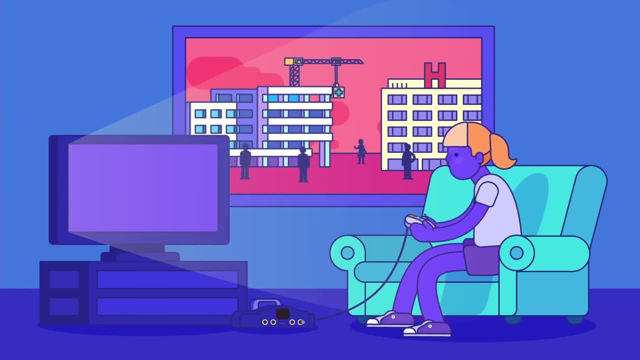 the rate of population growth will keep on slowing. This is true for every country In the West. we tend to overlook progress in other regions, but actually most of the world's countries have made it to the fourth stage. Just look at Bangladesh. 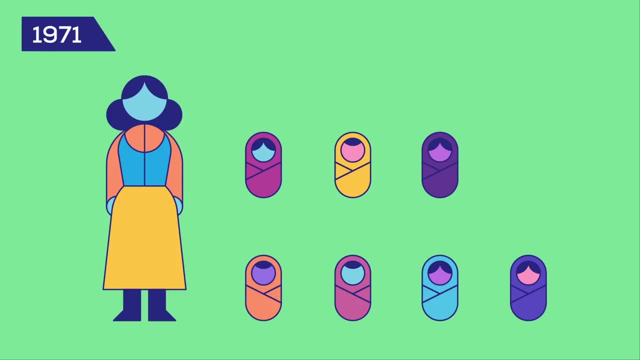 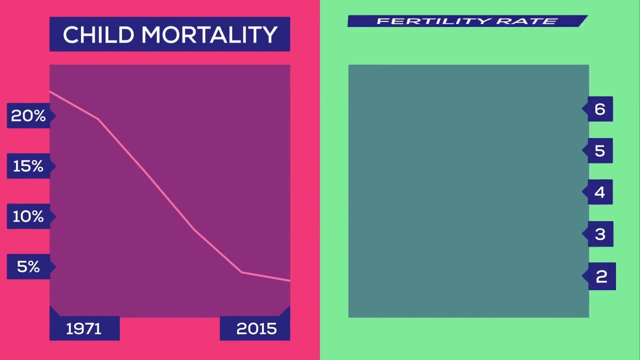 In 1971, the average woman had seven kids, but 25% of them would die before the age of five. In 2015,, the mortality rate was down to 3.8% and women had only 2.2 kids on average. 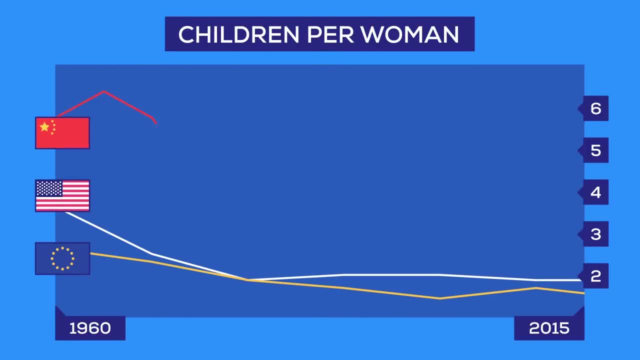 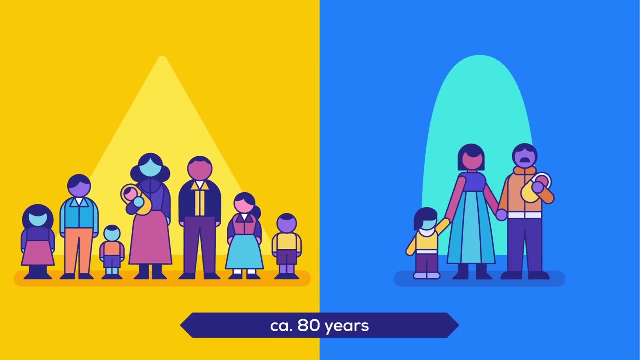 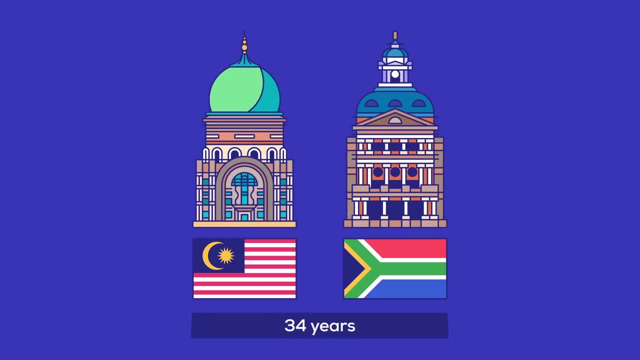 This is the rule, not an exception. We're not special, We just had a head start. It took developed countries about 80 years to reduce fertility from more than six children to less than three. Others are catching up fast. Malaysia and South Africa did it in only 34 years. 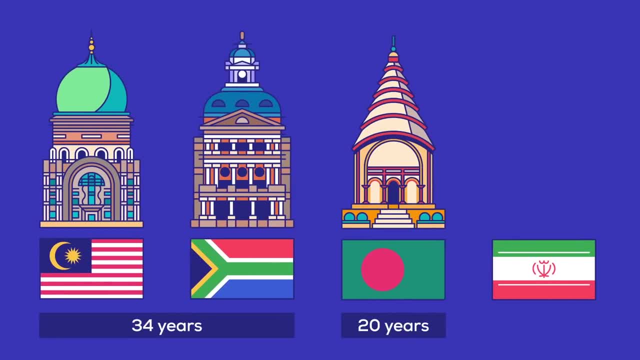 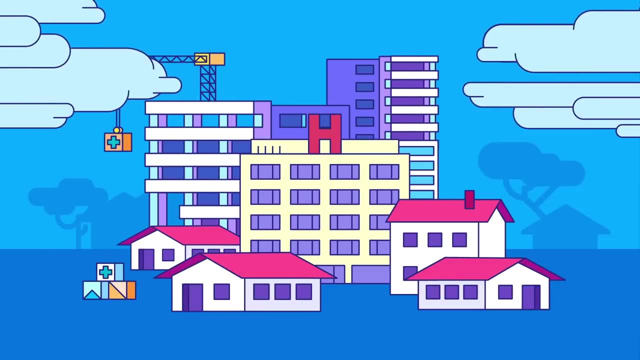 Bangladesh took just 20.. Iran managed it in 10 years. All these countries that are catching up didn't have to start from scratch, and the more support they get, the faster they catch up. This is why programs that help lower child mortality 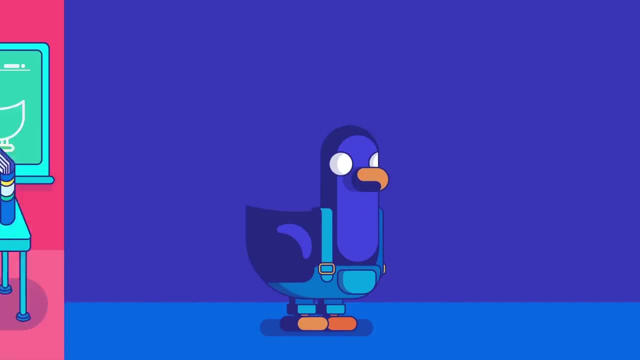 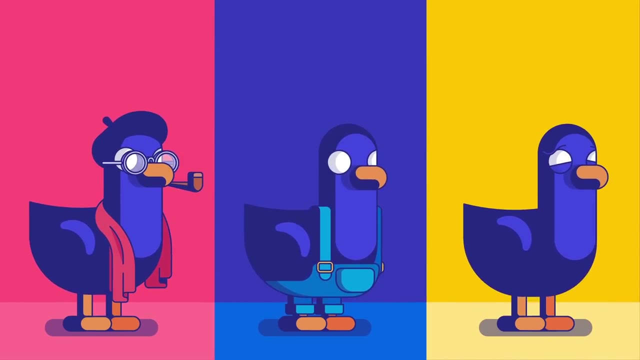 or help poor nations develop are so important. No matter what your motivation is- whether you dream of a world where all people live in freedom and wealth, or you just want fewer refugees coming to your country- the simple truth is that it's beneficial to you personally. 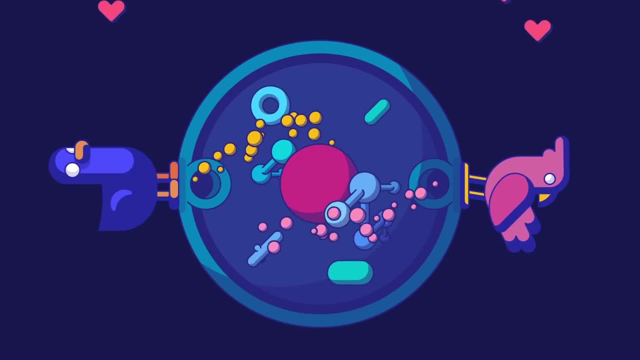 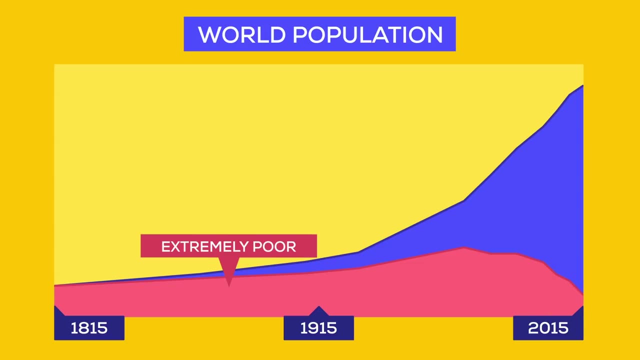 if people on the other side of the globe can live a good life. And we are getting there. The percentage of people living in extreme poverty has never been as low as today, So the future of global population growth is actually not an apocalyptic prophecy at all. 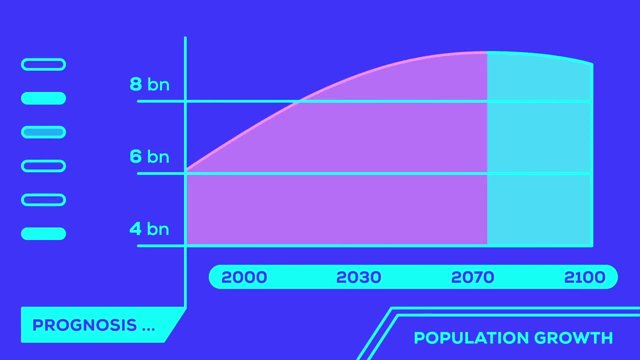 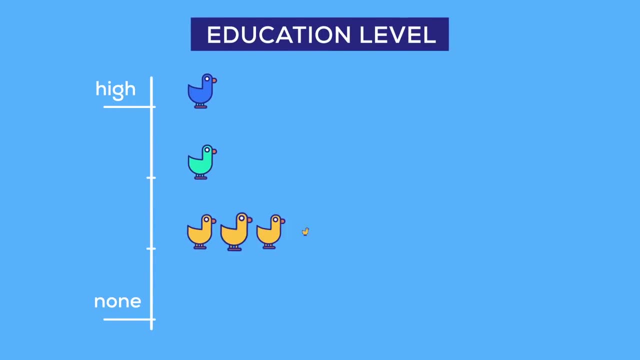 It's a promise: Population growth will come to an end. The UN forecasts that the 12th billionth human will never be born at all, And as the development level of the world rises, the number of people with a higher education will increase tenfold. 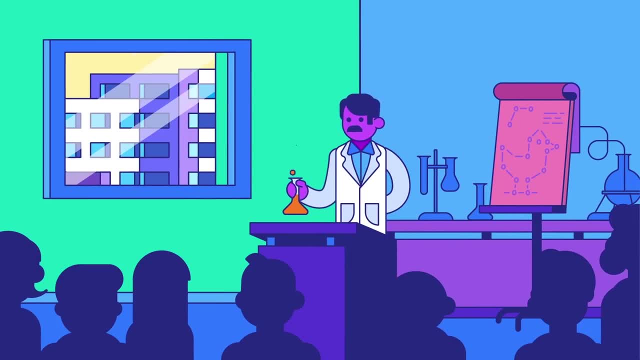 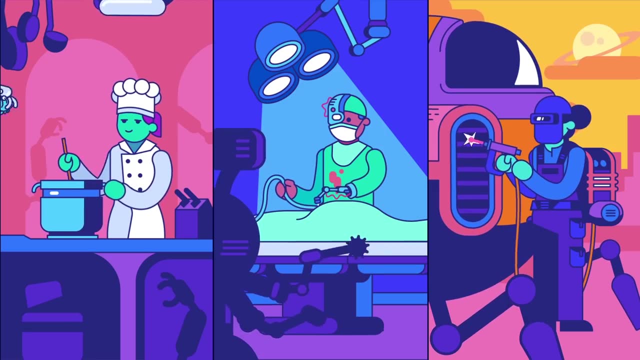 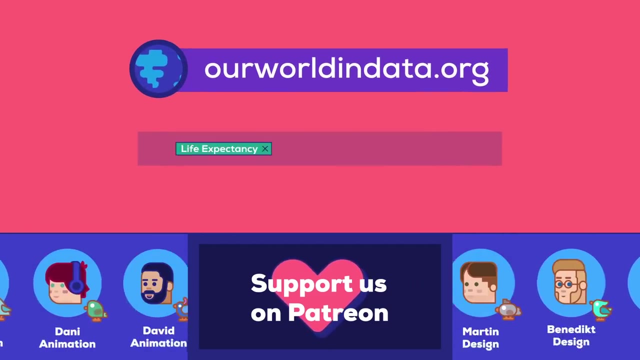 Countries who used to be in need will help advance development. instead. More people is going to mean more people able to advance our species. This video was a collaboration with Max Rosa and Our World in Data, where he explores the progress of humanity through research and data visualization. 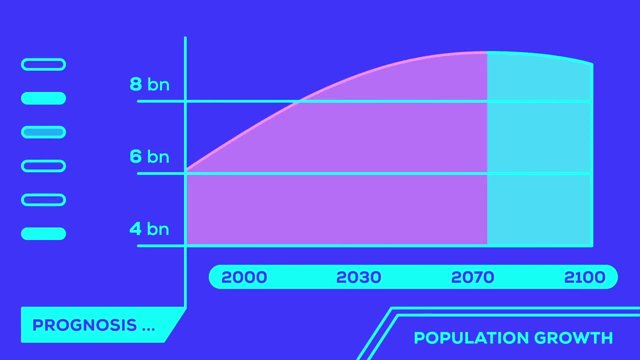 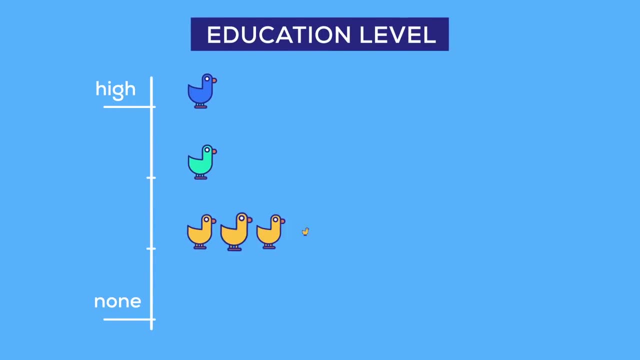 It's a promise: Population growth will come to an end. The UN forecasts that the 12th billionth human will never be born at all, And as the development level of the world rises, the number of people with a higher education will increase tenfold. 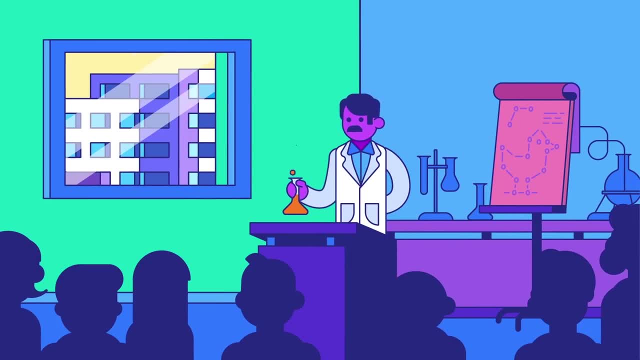 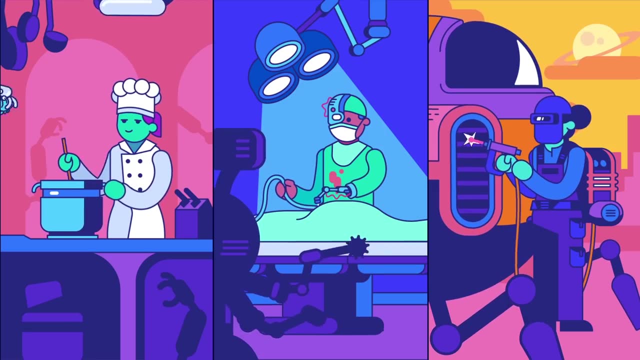 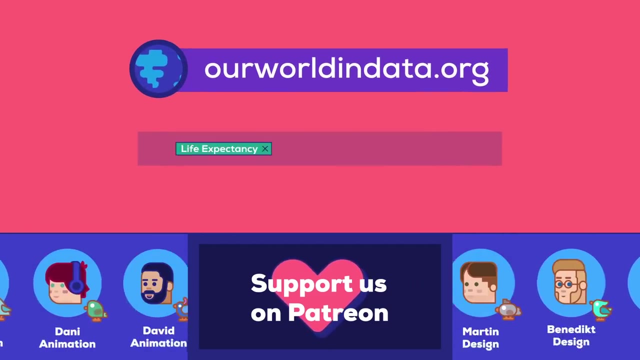 Countries who used to be in need will help advance development. instead. More people is going to mean more people able to advance our species. This video was a collaboration with Max Rosa and Our World in Data, where he explores the progress of humanity through research and data visualization. 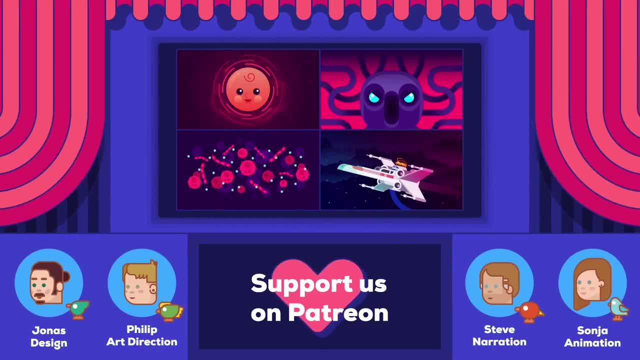 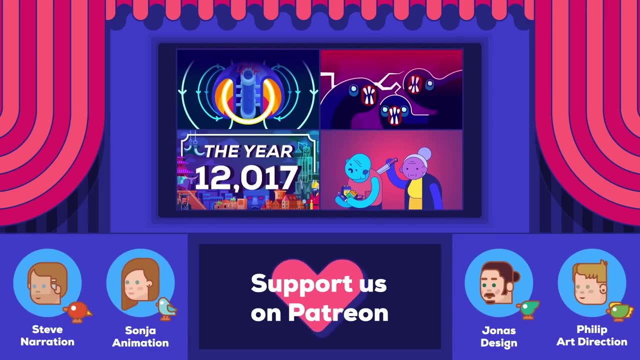 Make sure to check it out In 2016,. we were able to make more and better content than ever before because of your support on patreoncom. Thank you so much, And we'll be back in the year 12,017.. 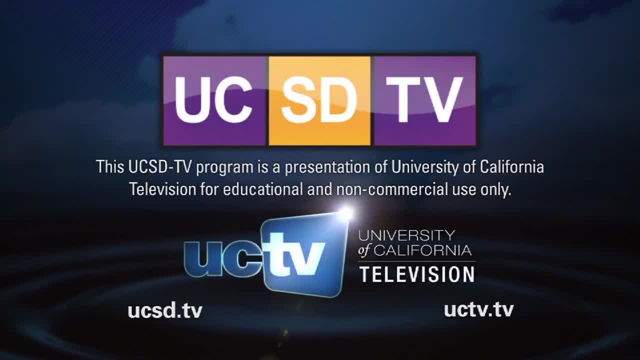 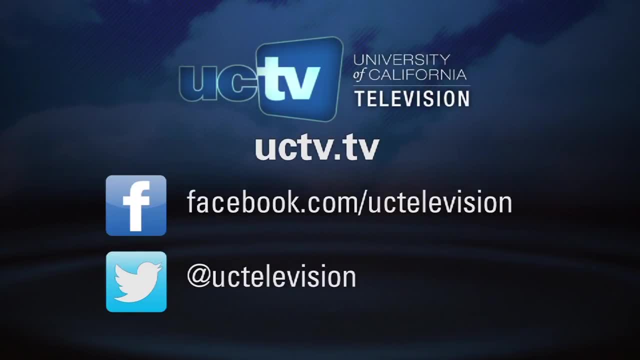 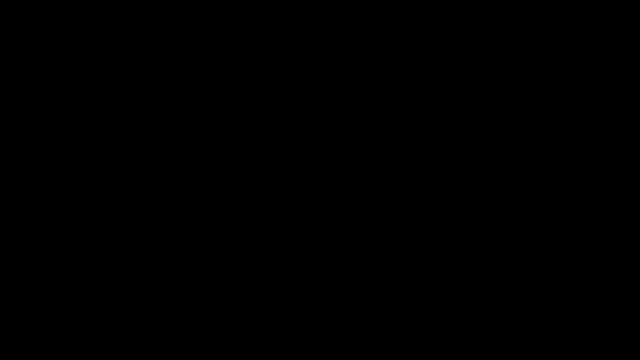 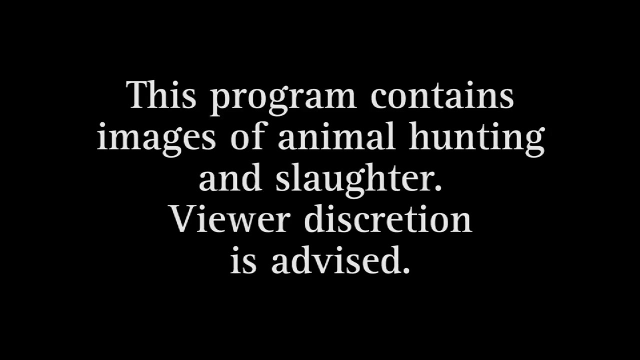 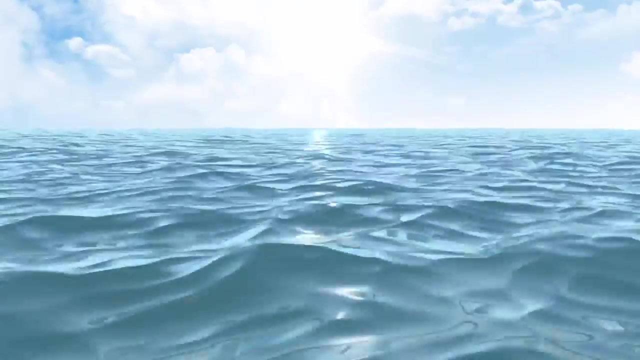 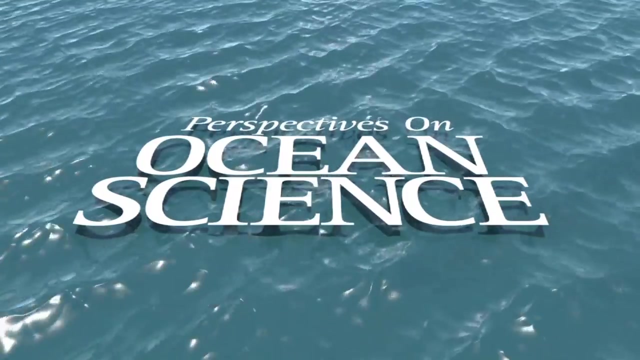 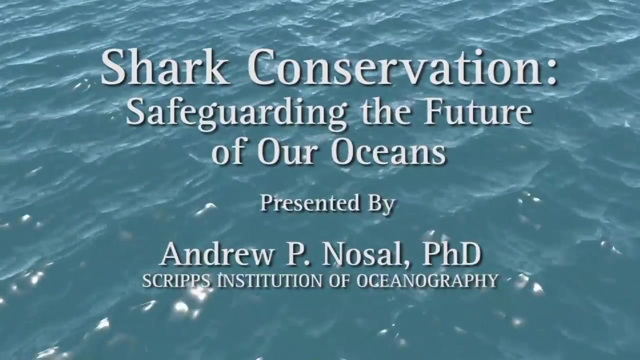 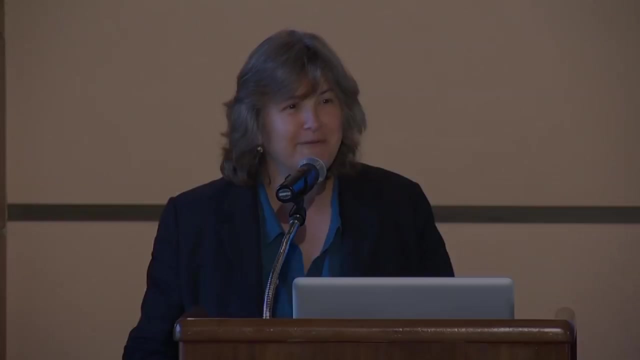 This UCSD TV program is presented by University of California Television. Like what you learn, Visit our website or follow us on Facebook and Twitter to keep up with the latest programs. Good evening and welcome to the Birch Aquarium at Scripps Institution of Oceanography at. 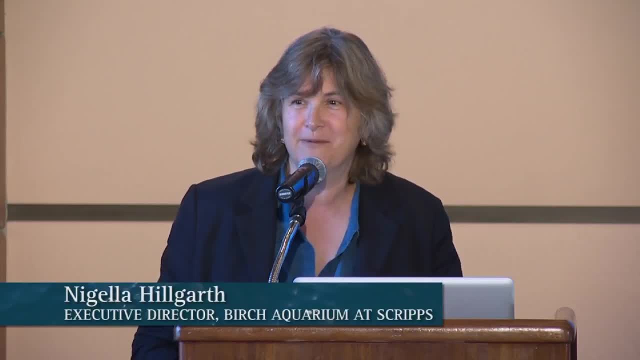 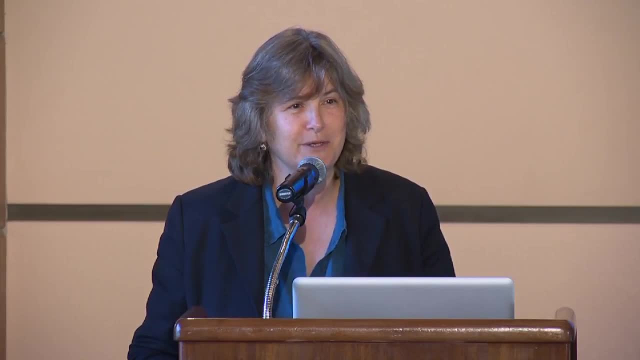 UC San Diego. My name is Linda. I'm the director of the Scripps Institution of Oceanography at UC San Diego. My name is Nigella Hillgarth and I'm the executive director here at the Birch Aquarium, and I'm delighted to welcome you to the latest Jeffrey B Graham Perspectives on Ocean Science.